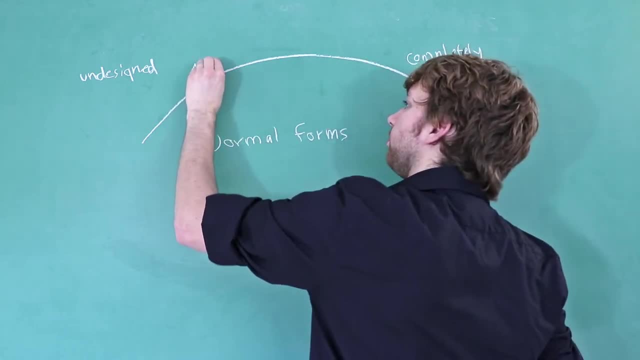 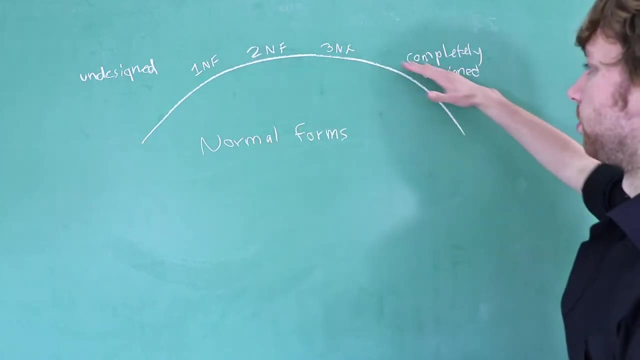 forms on this continuum. you would have first normal form, second normal form, third normal form, and then there's some extra normal forms down here which make the complexity a lot higher. So generally I like to stop here at third normal form, I think. 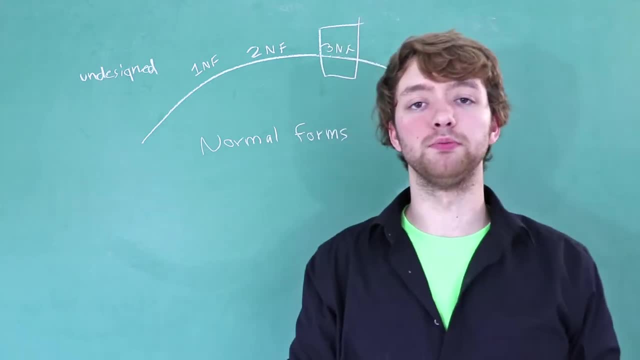 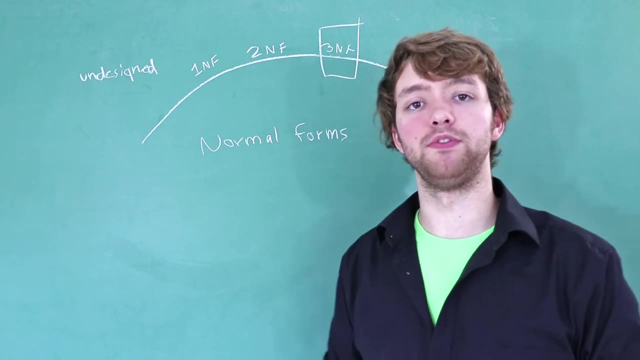 that's like the perfect place to stop, where your database is not too complex, but it's also extremely well designed to avoid bad data. So that's what we're going to be doing in the next couple videos: First, normal form, second normal form and third, normal form. Now I know I've been 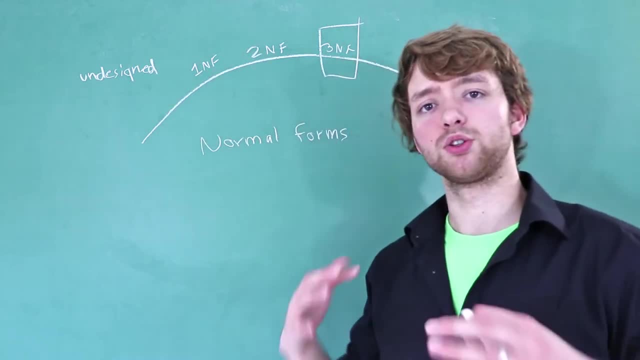 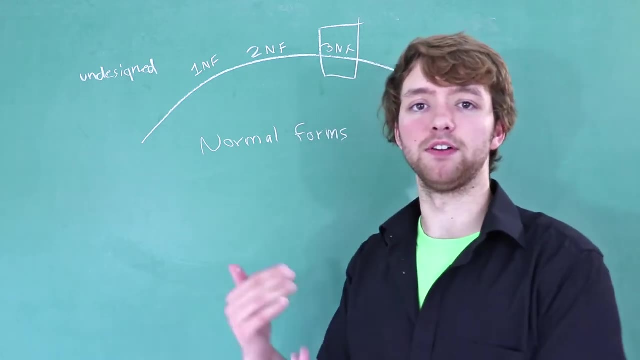 blabbering about these normal forms and I haven't really even explained them that much, but I'm going to explain them that well. So let's just start from the beginning with first normal form. What is first normal form? Well, it's the very first step of database design. Now make sure you watch the 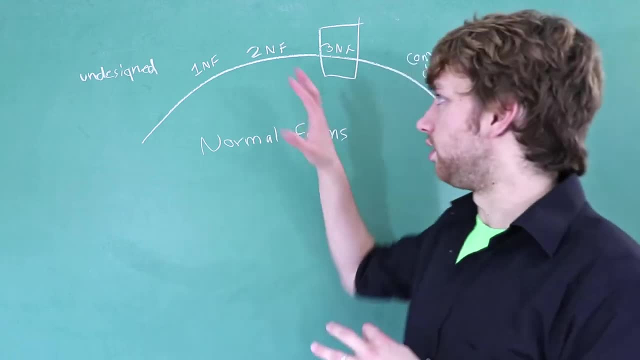 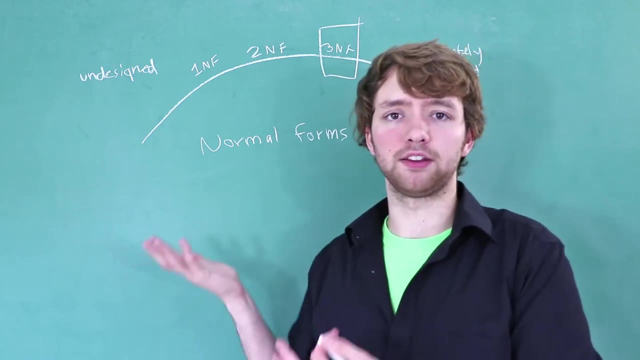 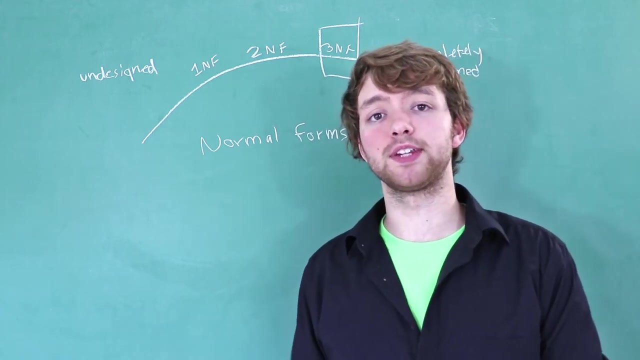 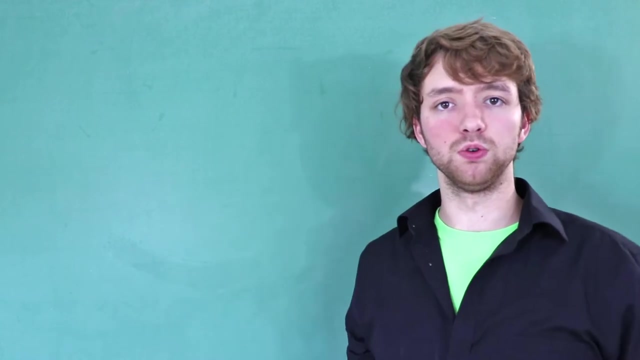 relationship videos and the previous videos, because the normal forms kind of build upon that and a lot of the problems with these normal forms are basically automatically fixed when you design your relationships properly. Not everything is going to be perfect, but if you get the relationships right it's going to be perfect. So let's get started. First, normal form has some rules that we need to. 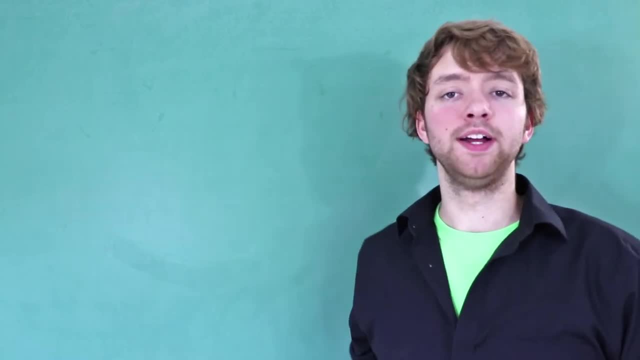 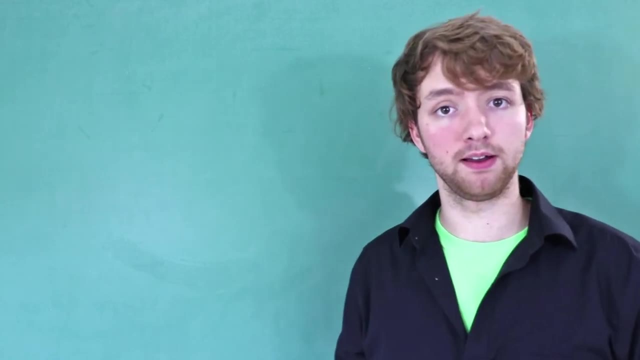 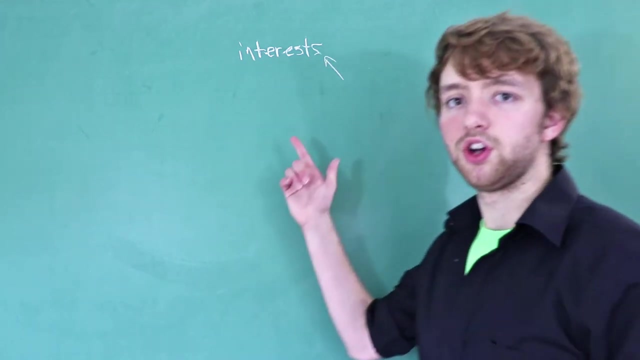 follow. The first rule is that every column in a table describes only one thing. The next thing is that every value for that column contains only one piece of data. So if we had a column interests, this is like a dead giveaway because it's plural. So this does not meet rule one. So rule number one: 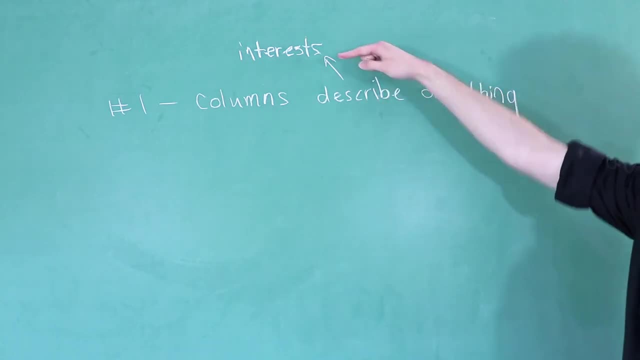 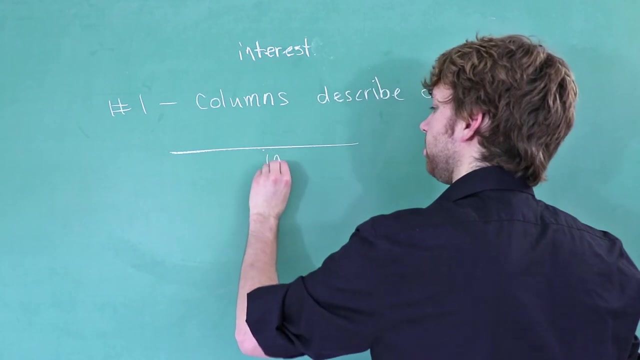 columns describe one thing. This is breaking that rule. So let's say we try to fix that and we just make it interest. So now we have this table and one of the columns in here is interest. So we have a users table and we're only allowed one interest. 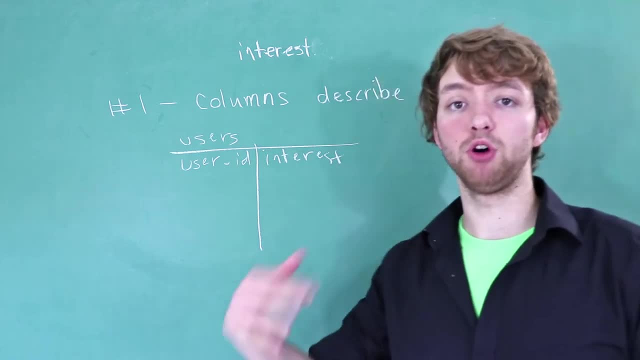 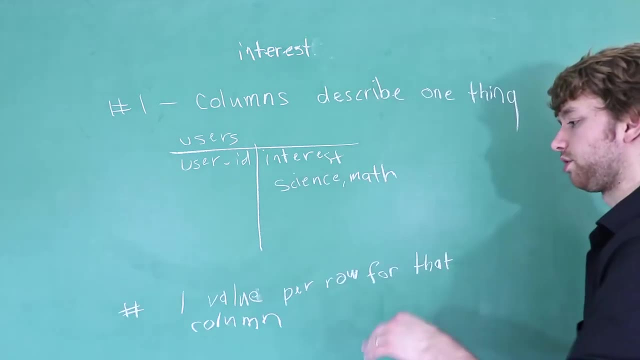 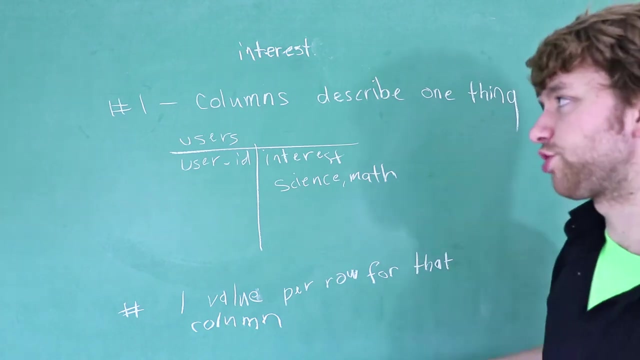 here. Well, let's say, someone you know goes in there and inserts multiple interests for one single column, just like that. Well, this is actually breaking rule two. So rule two essentially says there can only be one value per row for that column. And an additional rule is that 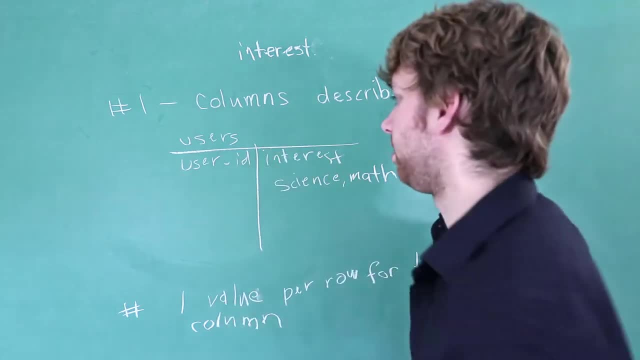 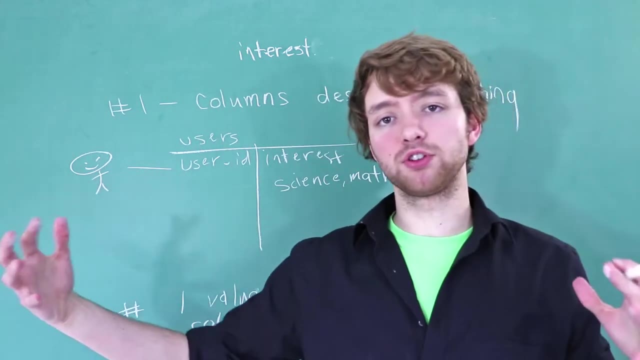 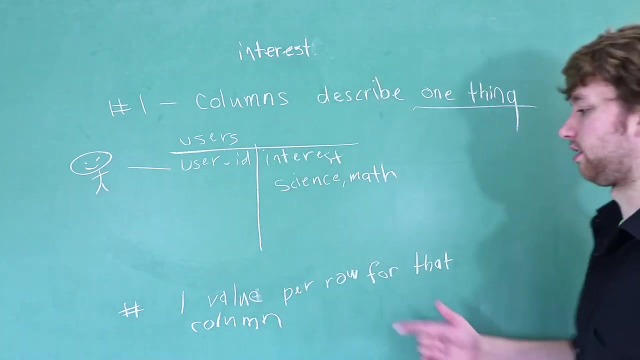 that you should only have one row per entity. So this refers to one specific user. So, essentially, if you wanted to encapsulate everything for first normal form, you would say: it follows the rule of one. So columns describe one thing. There's one value per row for that column and every single. 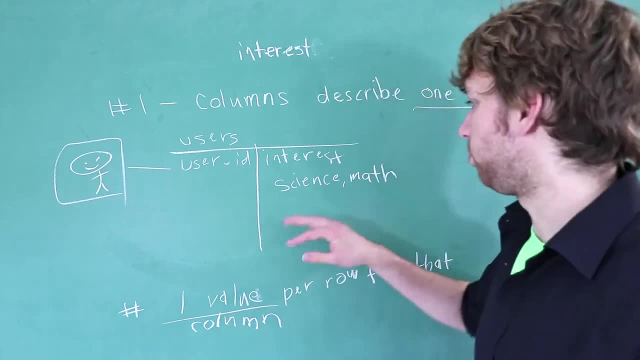 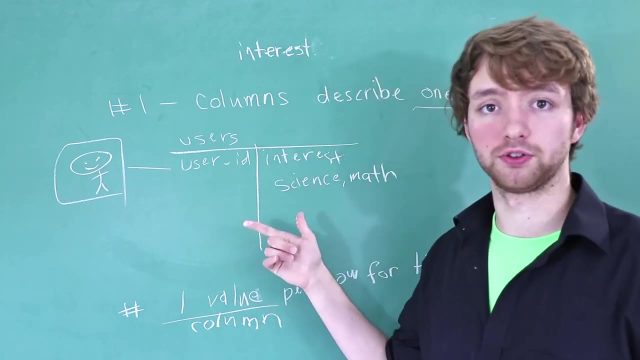 row describes only one entity. If you find that you want to store multiple interests or something in here, well, that's where I said the relationships are going to help you, because you'll understand how to structure that. A more common example that breaks first normal form is having a column name. 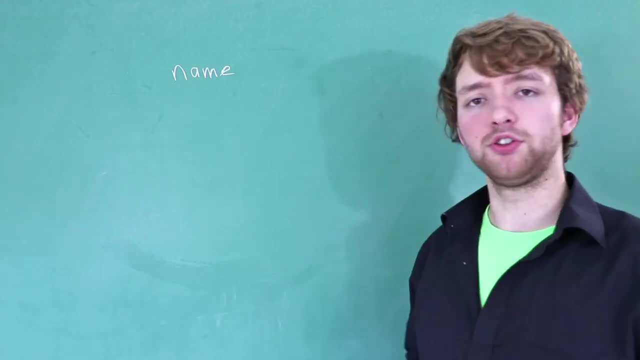 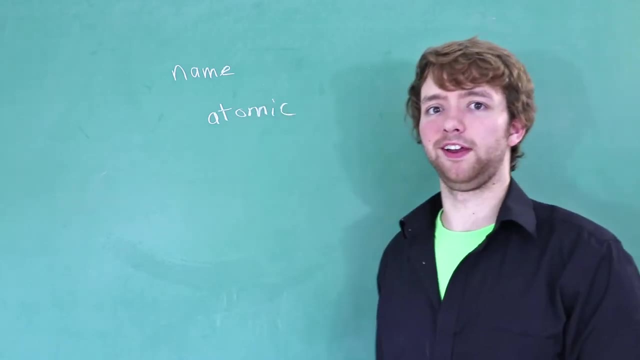 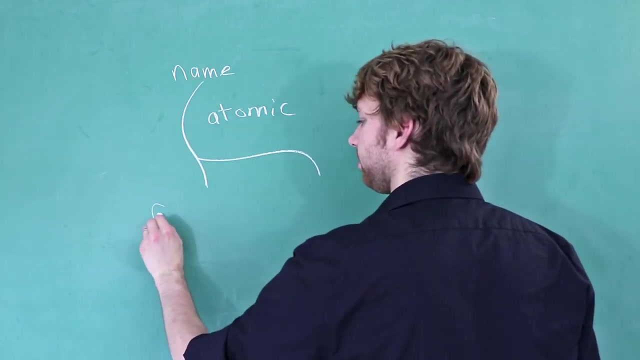 So name is that one thing. Well, the other term for being one thing is atomic, So think indivisible, because you know atoms can't be split, right? Okay, so this is really broken up into two things. We have the first name. 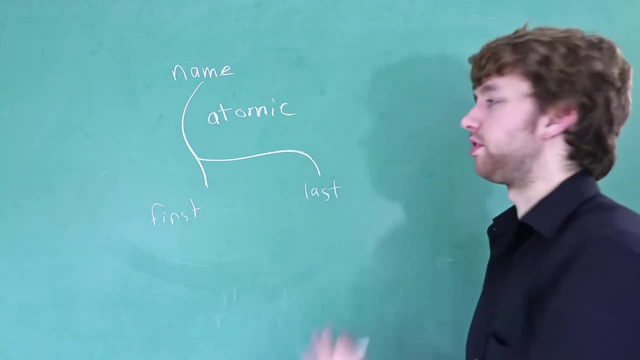 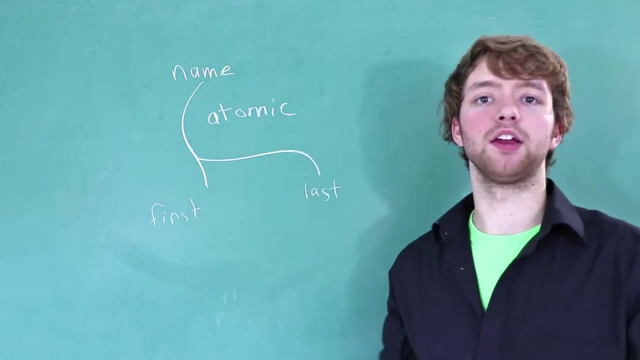 and the last name. This is an example that you might want to split up into two columns or three if you want the middle. Some people decide, hey, I'm just going to put in one column and we can't query by last name. 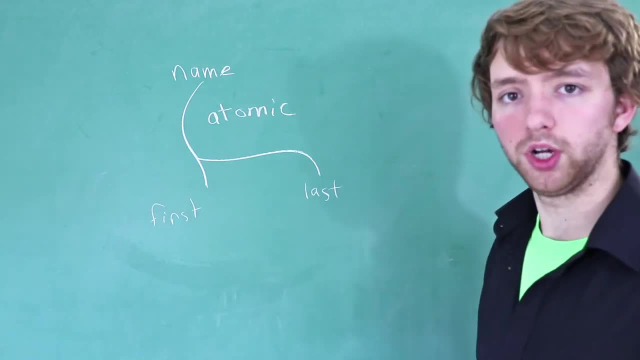 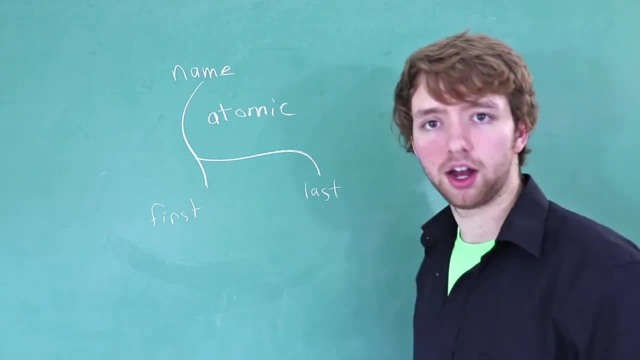 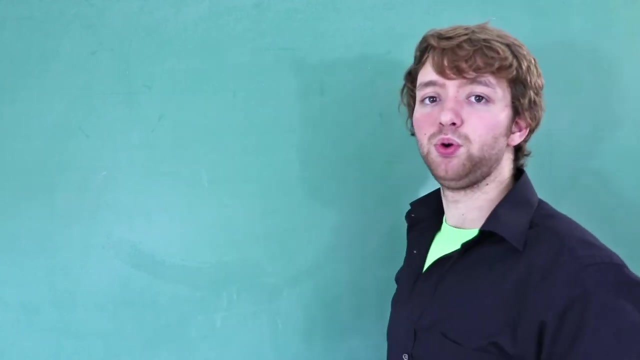 But if you break it up into first and last name, you can do queries saying like select everything from the users, where the user's last name is blah blah. That kind of thing is harder to do if you store the first and last name inside of one column. Another common example is the address: 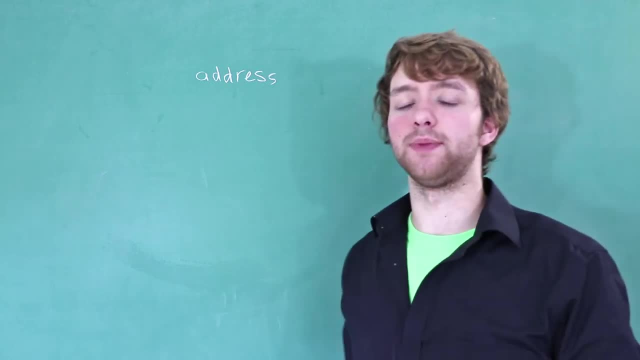 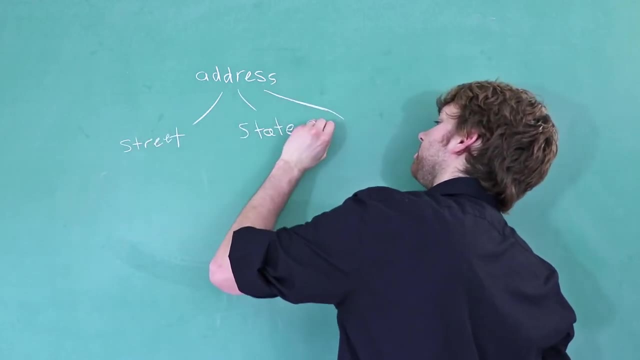 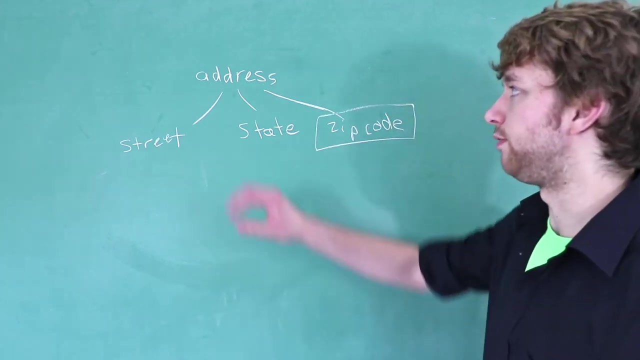 So the address is actually not atomic. If you think of what an address is, it's usually a street or a street number, a state and then a zip code. Well, if you wanted to get all of the data within a certain zip code range, it wouldn't be easy to do if you just stored one column address. 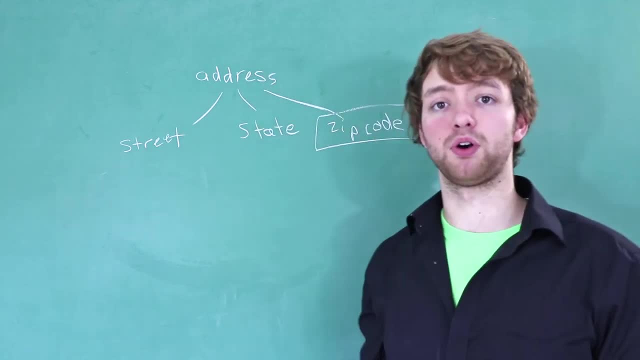 So you always want to try and break things up into the smallest pieces as possible. This follows the first rule that I mentioned of first normal form, where a column describes only one thing. So you always want to try and break things up into the smallest pieces as possible. This follows the first rule that I mentioned of first normal form, where a column describes only one thing. 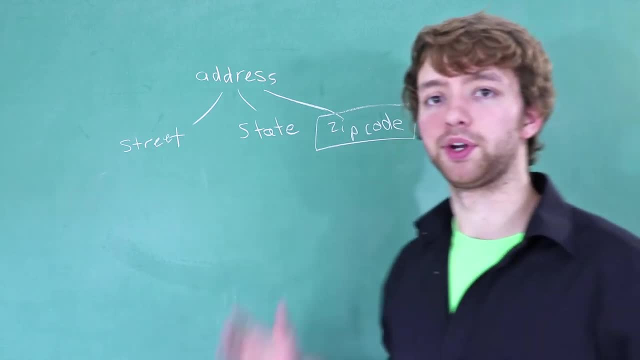 So you always want to try and break things up into the smallest pieces as possible. This follows the first rule that I mentioned of first normal form, where a column describes only one thing: A state and a zip code. Pretty good, If you want to extend that rule of one thing a little bit more to make your database really good.